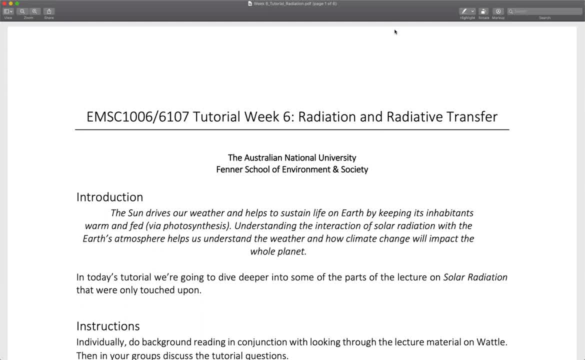 a great depth in this lecture on solar radiation. However, all the material I think you need to successfully complete this tutorial can be found in the lecture on solar radiation. Where I felt you might need some extra information, I've tried to include it in the questions here. 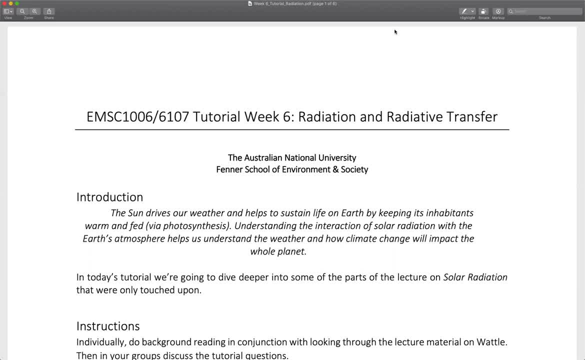 But if the lectures and what I've provided in the questions isn't enough, by all means do avail yourself of the wonderful resource that is Google. I'm not ashamed to say that I often refer to Google when I need some quick reference advice. 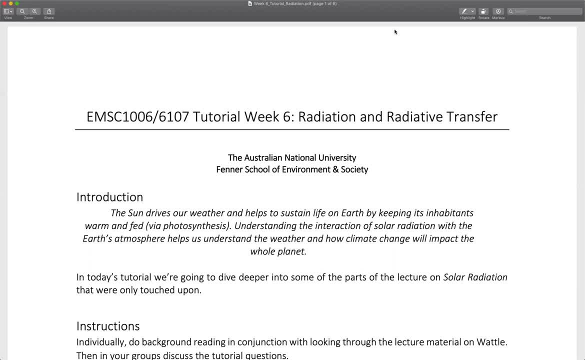 like: what's the gravitational constant, mean Earth-Sun distance, mean Earth's mean radius of the Earth, for example? So it's a great resource for that stuff, but don't trust everything, you see. And so I do suggest that, as far as authority goes, my lecture notes what I have here. and then, third, 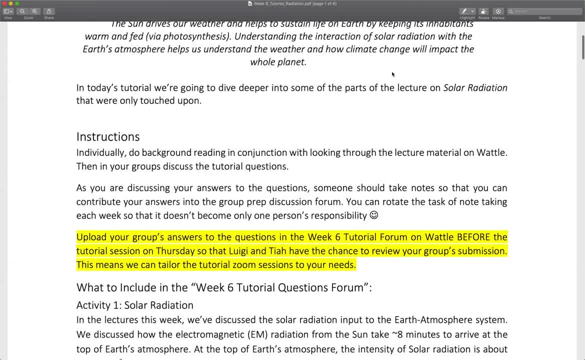